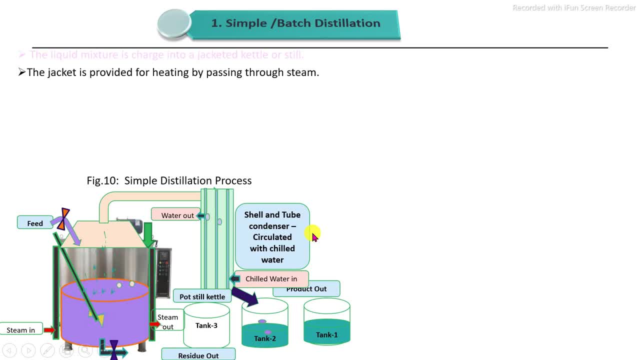 simple distillation process. the first, that is the liquid mixture, which is the charged into the distillation kettle. After that, if kettle is externally provided, or maybe heating is carried out by external heat exchangers or by providing the internal coil system, Then after that, whatever the liquid mixture, which is the continuously heated by circulating the steam to continuously boiling, resulting formation of the vapor. 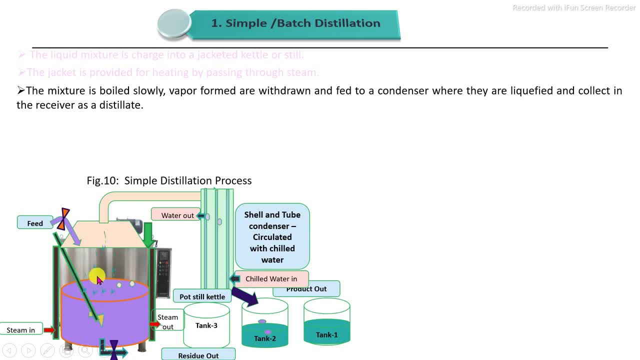 These vapors are formed, in which the continuing more volatile component, which are the pass into the condenser and then condensation process is occurred and finally we get the distilled product. With respect to the time of the distillation process, whatever the product which are get, in which the first initially product we get, the more concentrate, then its concentration is reduced with respect to the time. As per our requirement, we can collect the distillate into the fractions. that means first fraction, second fraction. 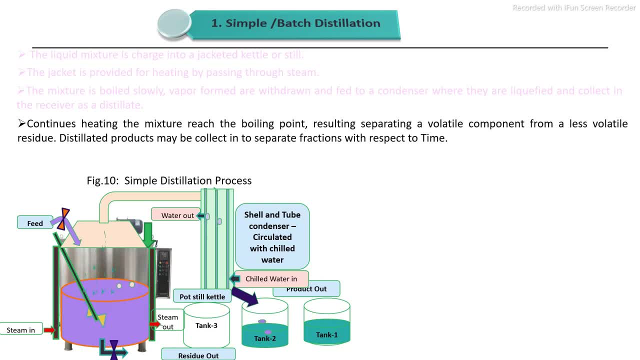 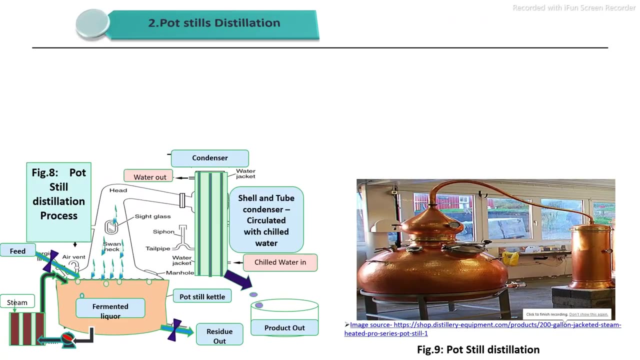 And the third fraction into this separate tank and this way, after the completion of the process, they deserve the, whatever the residue remaining, and then finally again wash and second batches operated. Secondly, the pot, still distillation. It is also simple type for batch, type distillation. The specific name is given here is: well, this is the pot which, in which 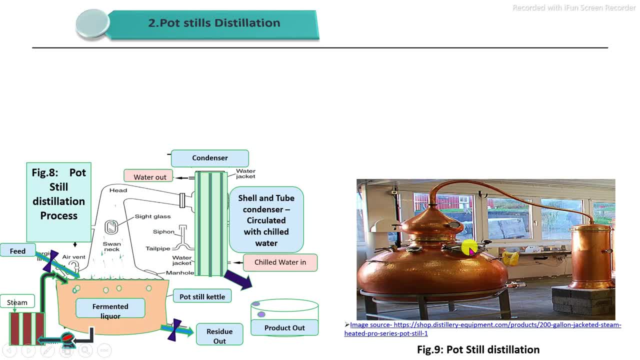 This is the pot in which pot is connected with the specific piping system, in which the swan neck like structure which is connected into the condenser. This type of the pot steel distillation is used in the whisky manufacturing processing, which is the constructed mostly in the copper tank. 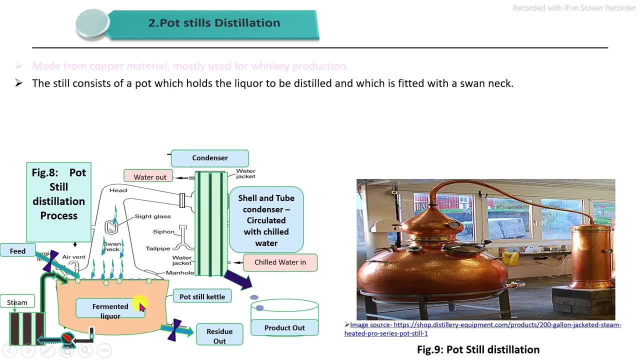 You can see the construction involving. first this is the pot. steel liquid mixture is heated by providing the external heat exchanger in which the formatted liquid is charged as per our required quantity. and this liquid is heated by circulating into the heat exchangers continuously, resulting heat transfer and start of the boiling of that formatted liquid. 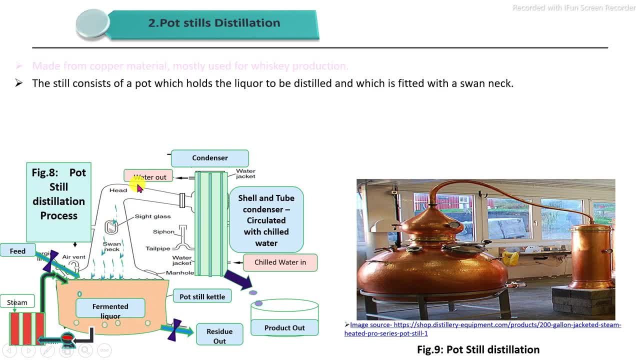 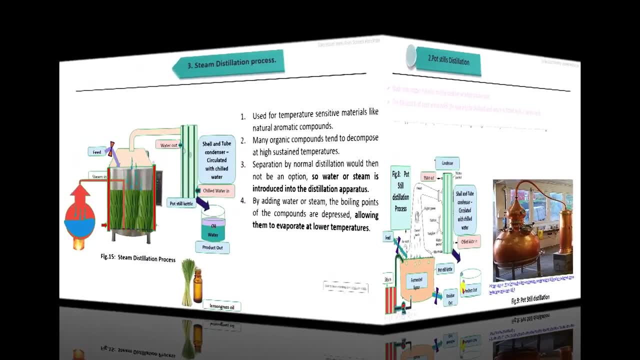 More volatile components, which are the released, which are then pass related to the liquid. So this is the pot steel distillation process, which is carried out into the condenser and the condensation process is carried out, resulting we get the distilled product. Next third one is the steam distillation process. 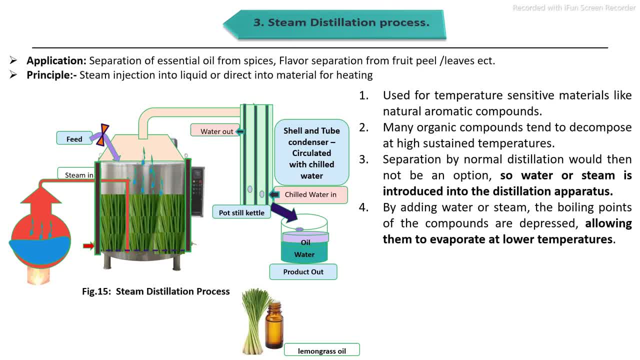 The steam distillation process. that means in which the steam is directly injected into the plant material, Mostly steam distillation used for the extraction of the essential oil from the plant materials in which the plant parts, mostly in which the maybe stem, leaves, flowers, etc. 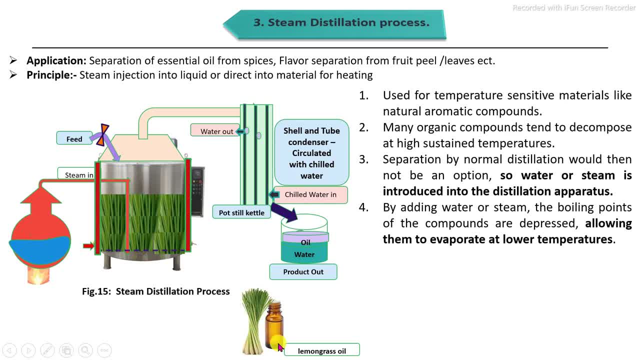 or maybe into the spices in the food processing industry, whatever the food peel containing essential oils which are the extracted by the steam distillation, or whatever the spices that containing essential oils which are the extracted by the steam distillation process, in which the first steam is formation separately in the boilers, which is the superheated steam. 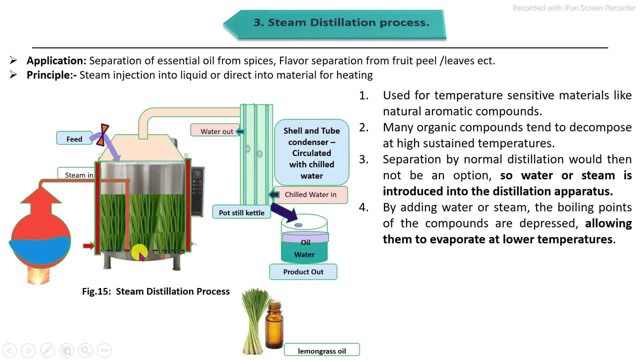 which is directly inject into the steam distillation system. There should be The Provision in which the whatever the plant materials- these are the- loaded into the perforated sieve and at the bottom, steam is directly injected, resulting whatever the hot steam which is directly contact with the plant material and it's containing moisture and volatile. 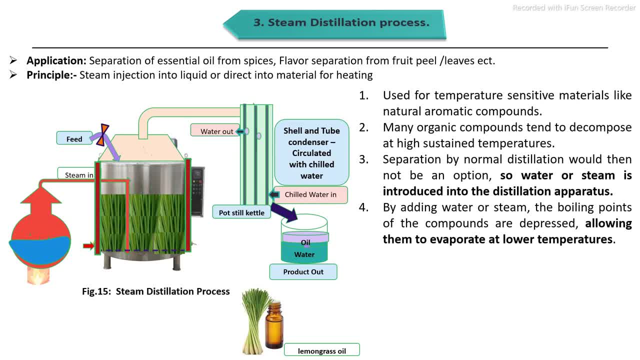 substance, which are the vaporized after the evaporation process. whatever the vapors, these vapors are condensed into the condensers and resulting we get the essential oil plus water. this, these are the component in which the oil, that is, the essential oil, which is the separated from the water by the separating funnels, and finally get the essential oil. 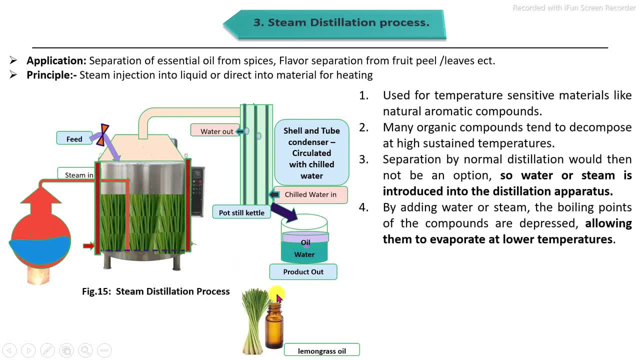 which is of the specific providing the flavor of that extracted material. the basic application is that some of the plant materials which are the more sensitive to the high temperature processing and the substances are released When We apply the direct steam injection system and the resulting we get. the specific oil substances are. 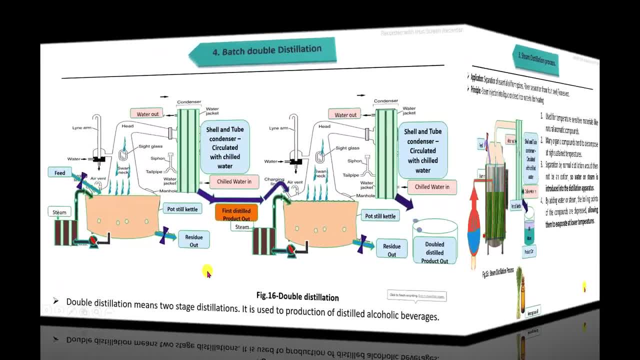 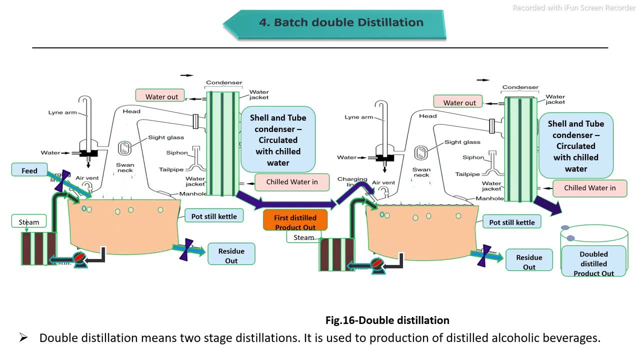 separation is carried out by the steam distillation process. batch double distillation, that means the batch a distributor which are operated into the series. that means you can see the two stage distillation process in which the first distillation, the formatted liquid, is charged into the first distillation and after